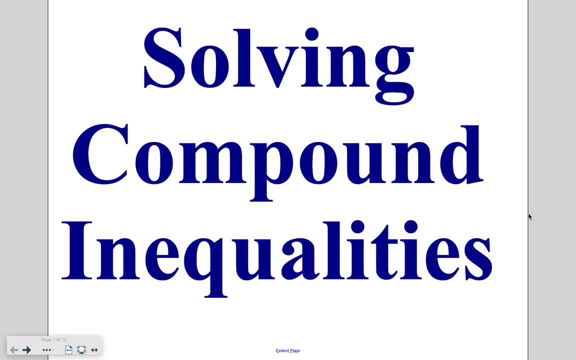 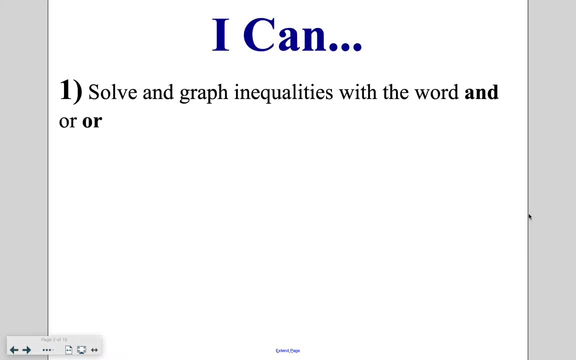 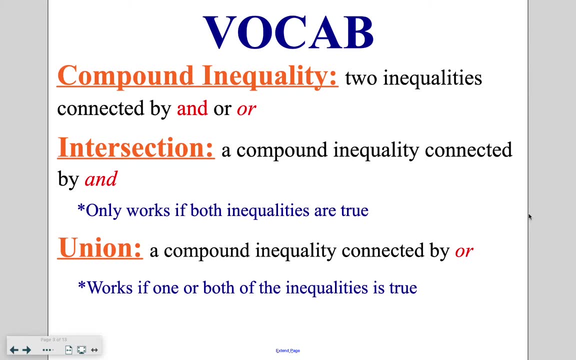 Hello class and welcome to today's algebra lesson, which is about solving compound inequalities. By the end of today's lesson, you will be able to solve and graph inequalities with the word and or or, So a little vocab to start today's lesson. A compound inequality is two inequalities. 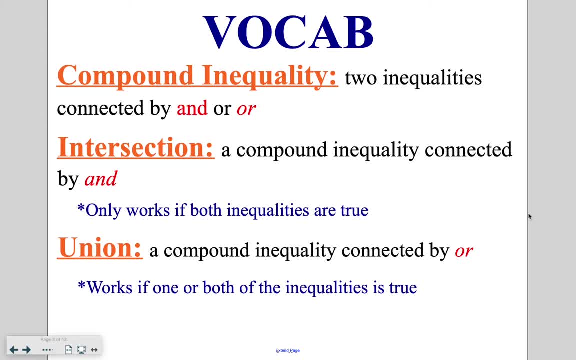 connected by the word and or or. If it is the first scenario, it's called an intersection. So these are the two inequalities that are connected by or. This only works, so when you're solving the problem and you get your answers, the statement only is true if both of the inequalities 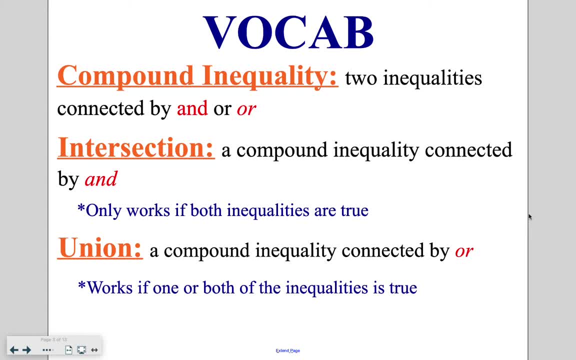 are true statements, So it has to work. the answers have to work for both parts. The second option is the union, which is a compound inequality connected by or. This means that the answers on the answer sheet are connected by or. If it is the first scenario, this means that the answers 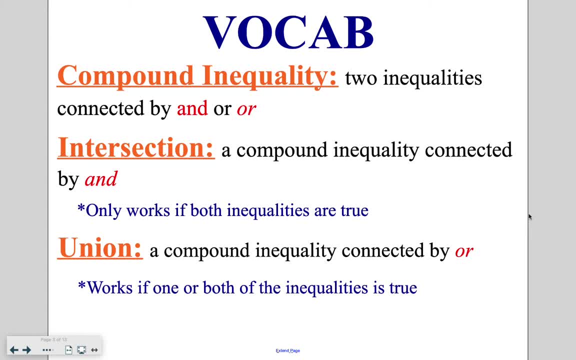 have to work for both parts. The second option is the union, which is a compound inequality Zeitung line only have to work for one or the other inequality. It does not have to work for both. It can work for both, but it only has to work for one or the other one. So we're going to start by 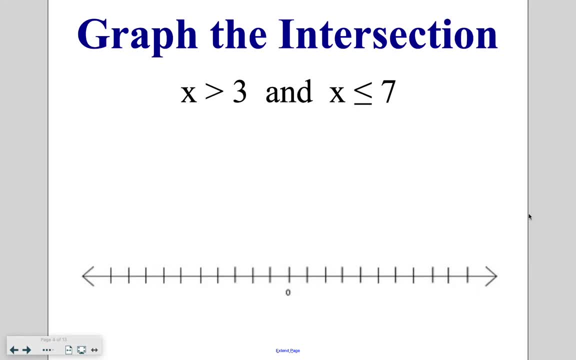 just looking at some basic ones. We're going to start with the intersection, So we're going to graph this. The statement says x is greater than 3 and x is less than- or, excuse me, x is less than 7.. So the first statement of x is greater than 3, I would start at 1,, 2, 3 and put my open dot. 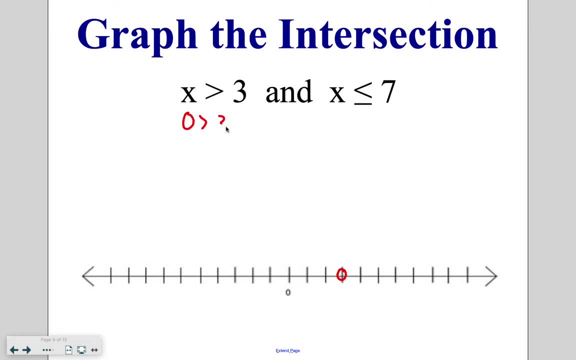 and then, if I test it, 0 is greater than 3 is a false statement. So I would be moving to the right and all of these answers are true for this first statement. So 4 is greater than 3,, 5 is greater than 3,, 6,, 7,, 8,, 9,, 10, etc. etc. etc. All of those numbers. are true for this first statement. So 4 is greater than 3,, 5 is greater than 3,, 6,, 7,, 8,, 9,, 10,, etc, etc, etc. All of those numbers are true for this first statement. So 4 is greater than 3,, 5 is greater than 3,, 6,, 7,, 8,, 9,, 10,, etc, etc, etc. All of those numbers. 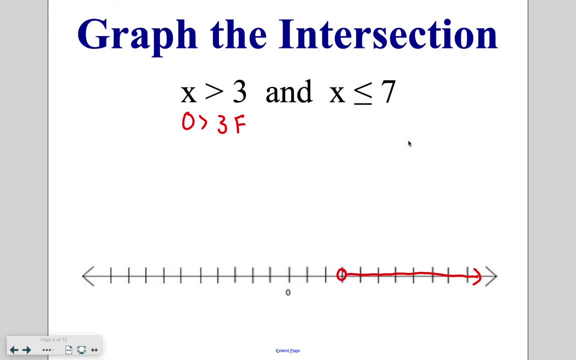 are true for this first statement. So 4 is greater than 3,, 5 is greater than 3,, 6,, 7,, 8, 10, etc. etc. etc. All of those numbers are bigger than 3.. Now what changes with this compound inequality is it says it also must be less than. 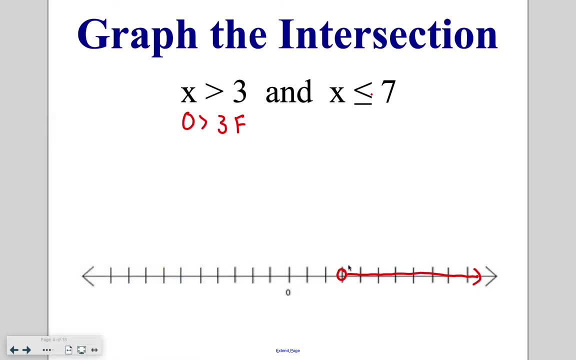 or equal to 7.. So I would come in and I would go 1,, 2,, 3,, 4,, 5,, 6,, 7 and I would put my closed dot. Then I've got 0 is less than or equal to 7, which is a true statement. So all of my answers for the 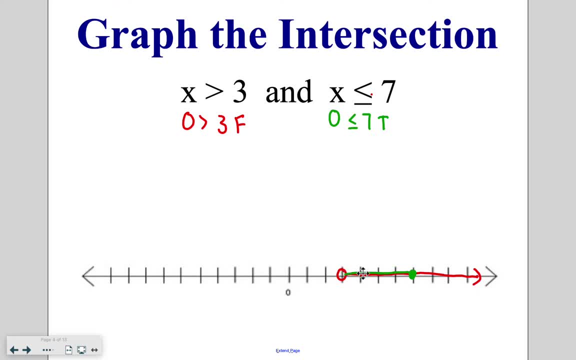 second one should be going to the left. However, we have to stop at 3, because none of the ones below 3 work for the first inequality statement. So what actually ends up happening here is these values above 7 are no longer part of our answer, So the only answers that work are between 3 and 7. 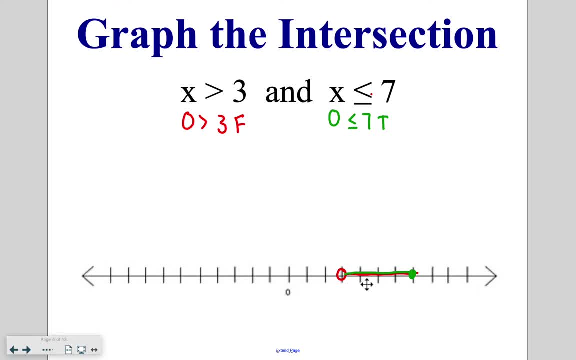 because this is an and statement. So 4 is bigger than 3 and it's less than 7.. 5 is bigger than 3 and it's less than 7.. 6 is bigger than 3 and it's less than 7.. So all of these, 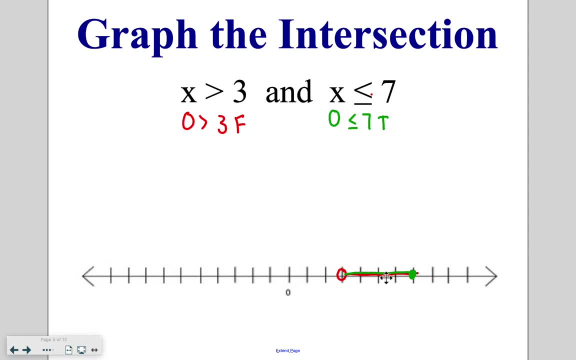 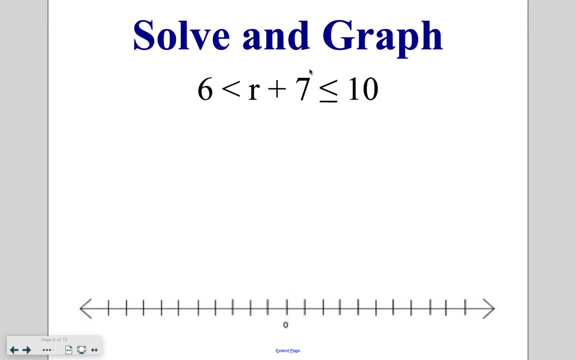 values on the inside of those two dots make up the answer for this intersection. You can also see intersections written as this one big inequality statement. So this is read as: 6 is less than r plus 7,, which is less than or equal to 10.. When: 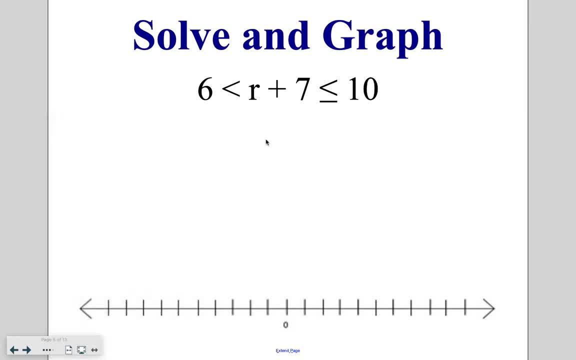 you solve this version if you take away 7 from the middle. so between the two inequality signs, you have to take away 7 from both of the outside values. so our final statement: that becomes negative. 1 is less than R, which is less than or equal to 3. the nice thing about writing it this way is it tells you exactly what. 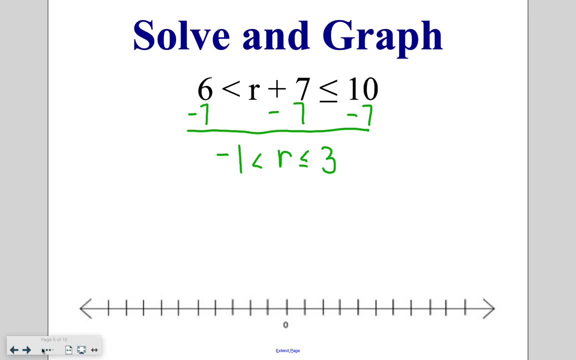 you are in between. so I would go to negative 1 and I would put my open dot at negative 1 because there is no equal to part there. so I've got my open dot- oopsies- at negative 1, not negative 2. and then I go to the right- 1, 2, 3 and put my 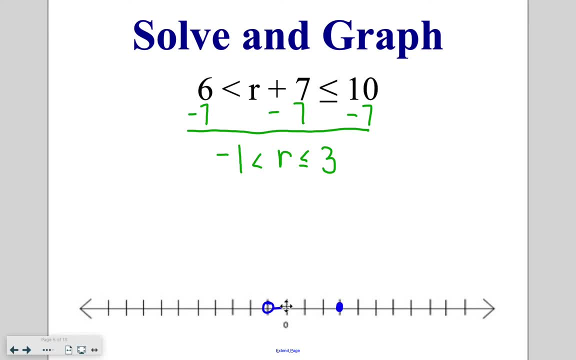 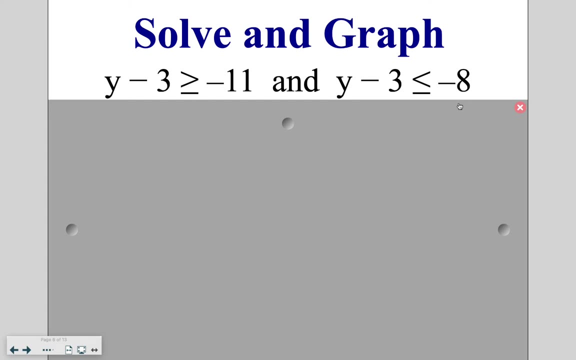 filled in dot and then my answers for this compound inequality are between those two dots, so all the values between negative 1 and 3 work for this answer. you can also see inequalities with the intersection written separately, where you would have to solve them both like normal cases. so I want you to go ahead. 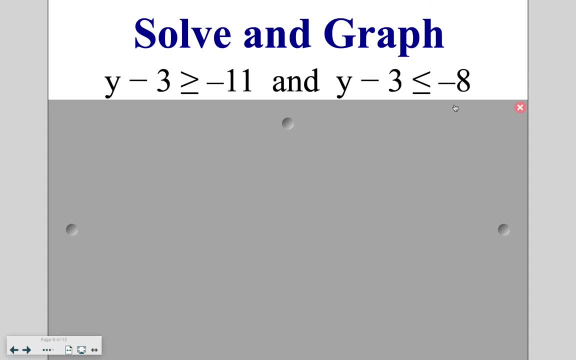 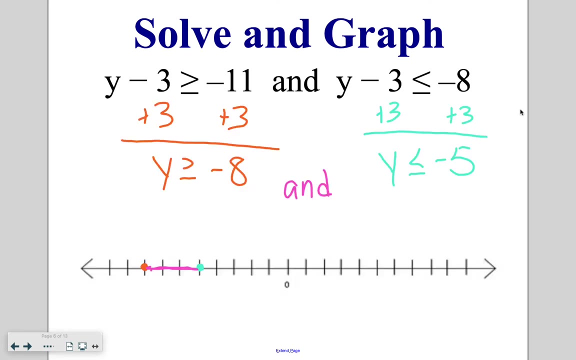 and solve this one on your own, telling me the two answers for the inequalities, the two dots that you would get and then where you would, where you would draw in that answer portion of the graph. so your first answer is: Y is greater than or equal to negative 8, and your second answer is Y is less than or equal. 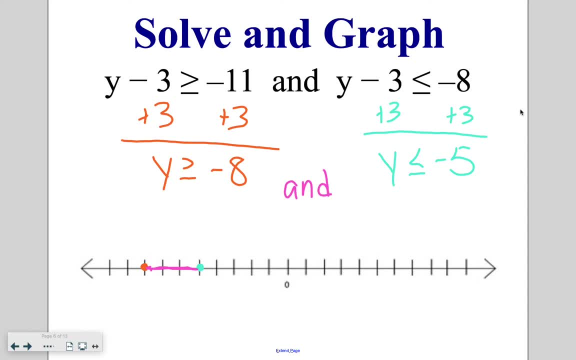 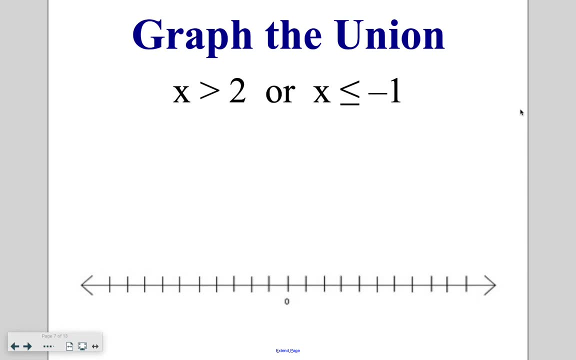 to negative 5. so it should have been both closed dots and the answers are between those two dots. moving on to the union now, this is the part where it has to satisfy one or the other. so, starting with the basic one, I've got. X is greater. 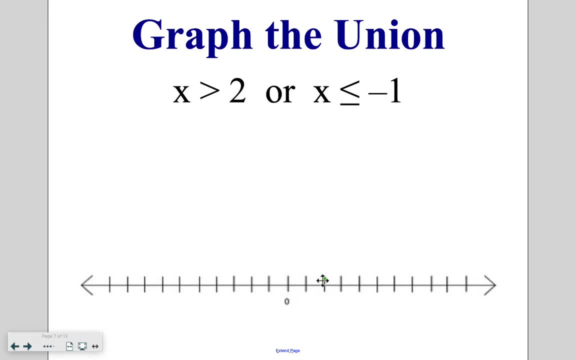 than 2. so I'm going to go to my graph and I'm going to put my open dot at 2. 0 is greater than 2 is a false statement. so we are looking for the values going to the right, all of those that are bigger than 2. for the second one, I've 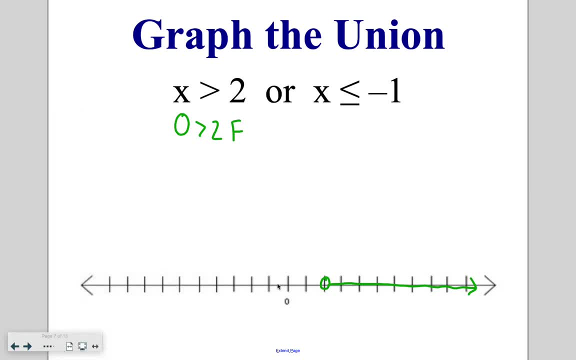 got that X is less than or equal to negative 1, so I come over to negative 1 and I put a filled in dot. now I've got that 0 is less than or equal to negative 1, which is once again a false statement. so in this case we are moving to the. 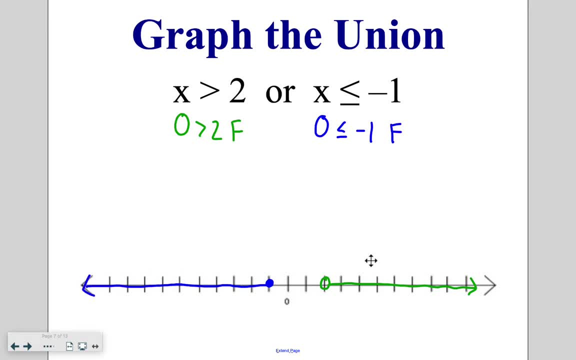 left. so what this means is that the green answers work for the first part but not the second one, and that's okay, because it only has to work for one. the blue answers work for the second part, but not the first part. again, that's okay, because it only has to work for one or the other. so this part we don't have to. 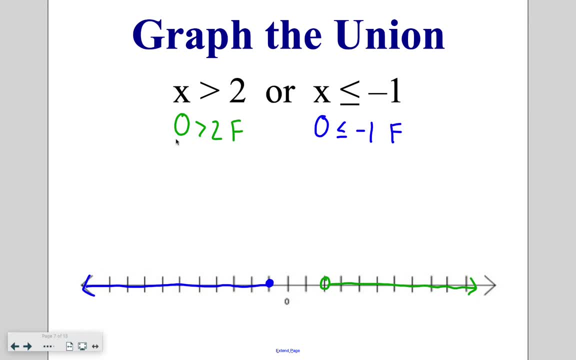 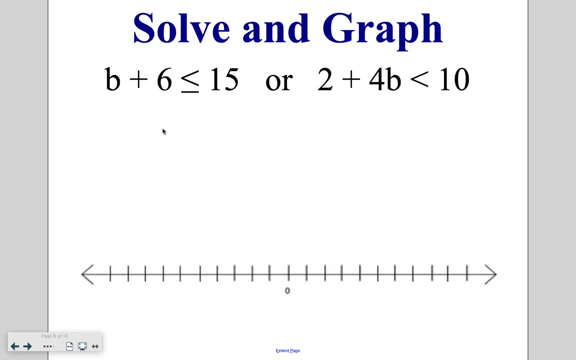 erase anything as we are on the graph, because it can work for one or the other. so now, when we get to solving these- this first one I've got- B plus 6 is less than 15. so I'm going to subtract 6 from both sides of my equation and I end up with: B is less than or equal to 9, so 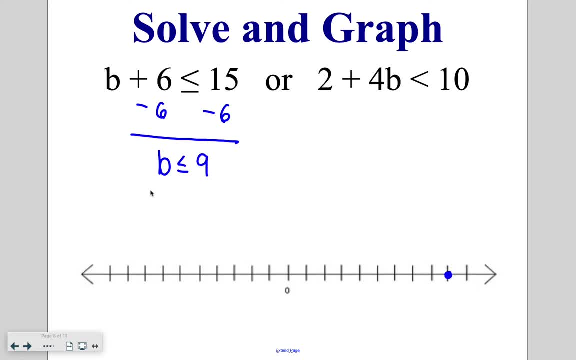 I'm going to start at 9 with a filled in dot and I'm going to test. my point of 0 is less than or equal to 9, which is a true statement. so I want all of those values going to the left which are smaller than 9 with my next statement. 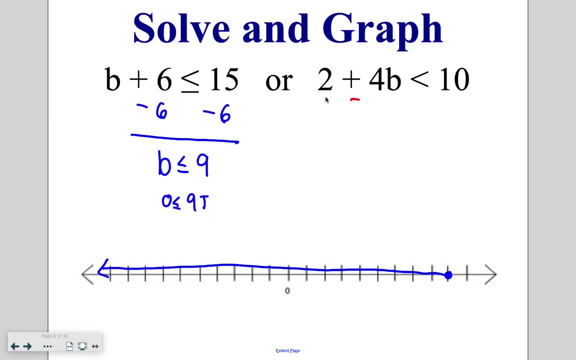 then I am going to subtract- excuse me, I am going to subtract 2 from both sides of my statement. so I have: for B is less than 8, and then I'm going to divide by 4 on both sides and I end up with B is less than 2.. so I'm going to come over to 2. 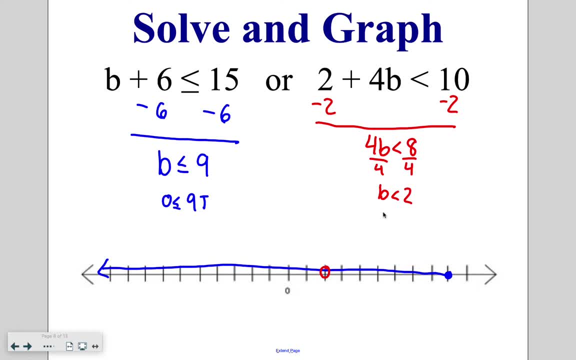 I'm going to put an open circle there and then I'm going to test a point. so 0 is less than 2 is also a true statement. so once again, I am moving to the left. so what this graph shows is that where the red and the blue overlap, that works for both, which is great, because it means it works for one. 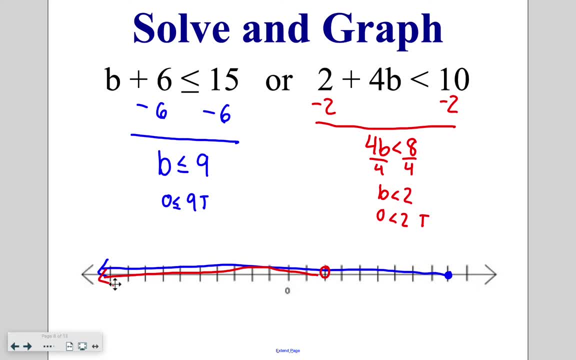 of them, where the blue is by itself, that only works for the first one and not the second one. again, that's fine, because it only has to work for one of them. and then this area up top where neither the blue or the red is. those are the numbers that don't work for either statement. 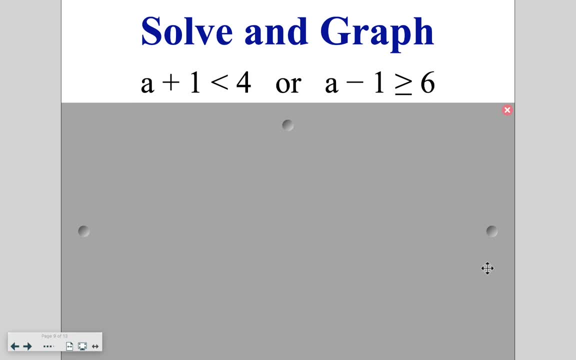 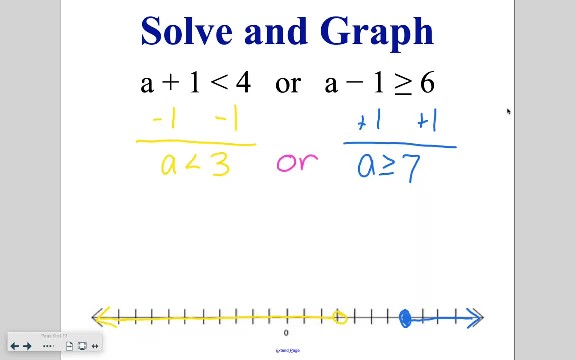 so go ahead and try this one on your own, saying the inequality, the dot and the direction for both statements. so when I solve the first one, I end up with a is less than 3, that's going to be the open dot going to the left. and when I solve the second one, I have a is greater than or equal to. 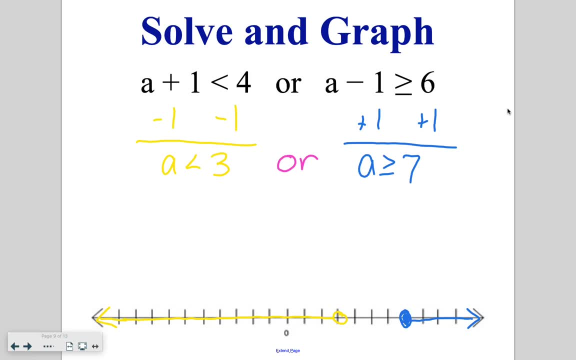 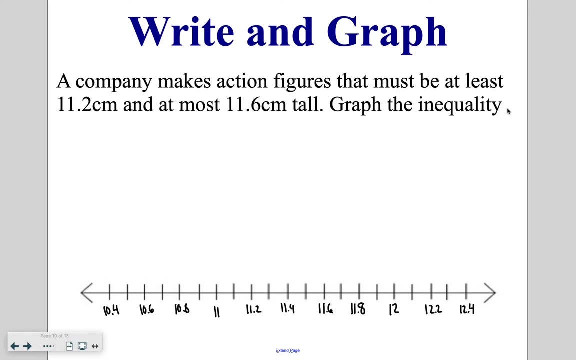 7, which is a closed dot going to the right when we have word problems. there's a couple different scenarios here. we have to decide if there are intersections, the and statements, or unions, the or statements. so I read the sentence: the company makes action figures that must be at least 11.2 centimeters and. 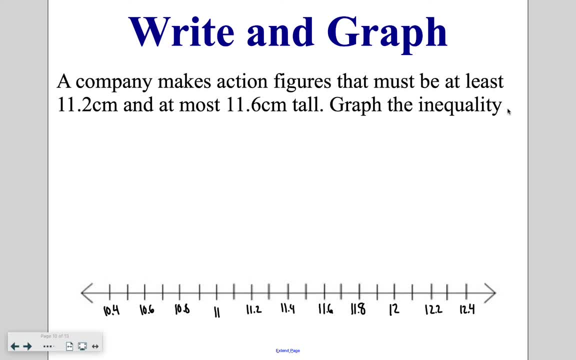 at most 11.6 centimeters tall. so the first thing we need to do is decide: are we trying to be between, with the and statement, between those two numbers, or outside of going either direction? so in this case, says it. says the first part is: I want X is at least so greater than or equal to. 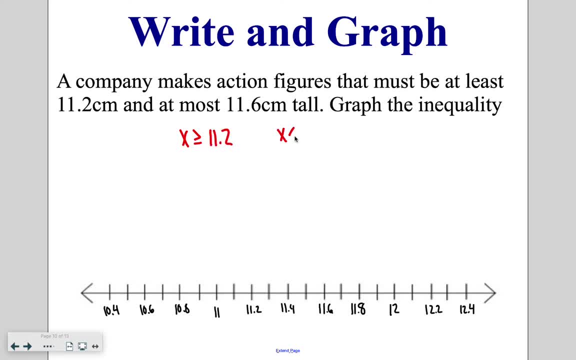 11.2 and we have X's at most, so less than or equal to 11.6. this is going to be an and statement, so you can write it as two separate pieces or, if you prefer, you can write it in that compound form for. 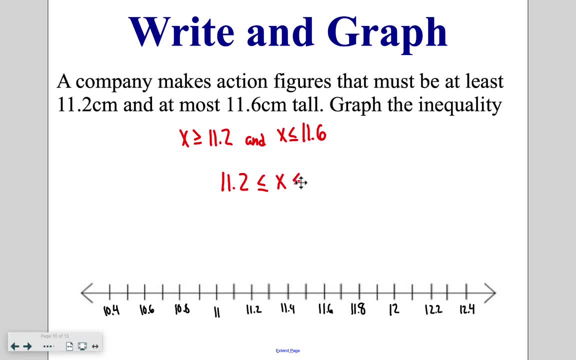 an and statement which is 11.2 is less than or equal to X, which is less than or equal to 11.6. now I'm going to come down to my graph and I'm going to put a close dot at 11.2, a closed dot at 11.6 and then connect them, because we are looking for those. 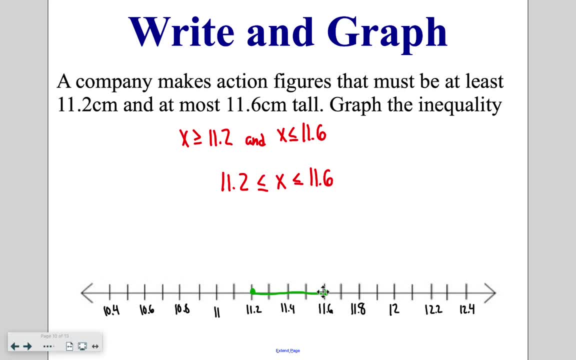 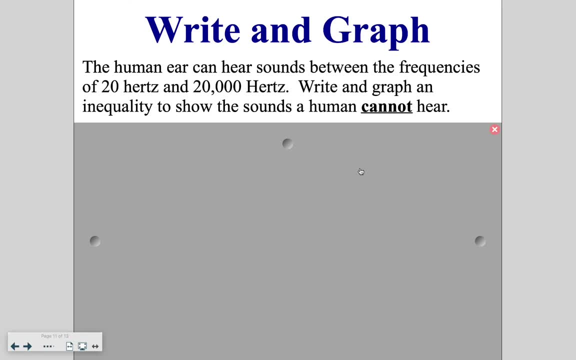 values in between those two points. go ahead and try this one on your own. first, I want you to just write the inequality. so when I write the inequality I have, X is less than 20 on the low end, because that's outside of what we can here on the low end. or X is greater than 20 000.. that's going to be the upper end of the problem. 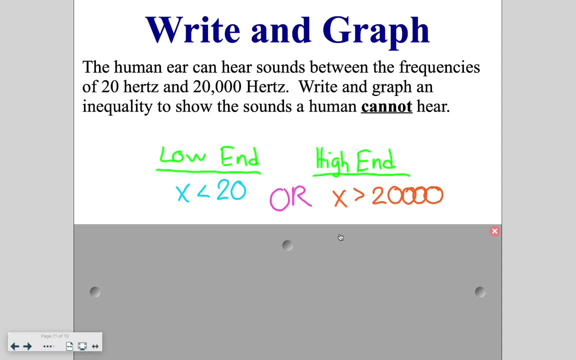 now explain to me how you would graph this inequality. so on the left side we have an open dot at 20 and the values are moving to the left smaller than 20.. on the right side we have an open dot once again and it is moving to the right. final piece here. if 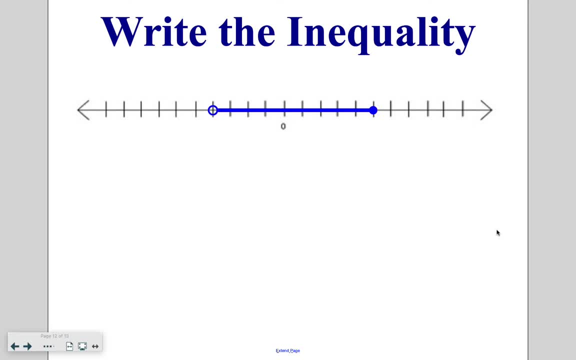 they give you the inequality and you need to- or excuse me if they give you the graph and you need to write the inequality. when we do this, we want to treat each side of the graph as its own separate piece. so when I look at this first part, I am one, two, three, four below zero, so I'm at negative four. 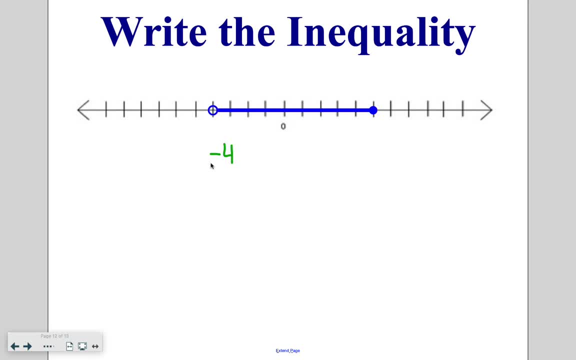 and my values here from this line are getting bigger than negative four. so my first one, I've got X- is greater than negative four because it's between- this is going to be an and statement. and then on the second one, I'm at one, two, three, four, five and those values are going to the left, so smaller than five. so I've got X is less.